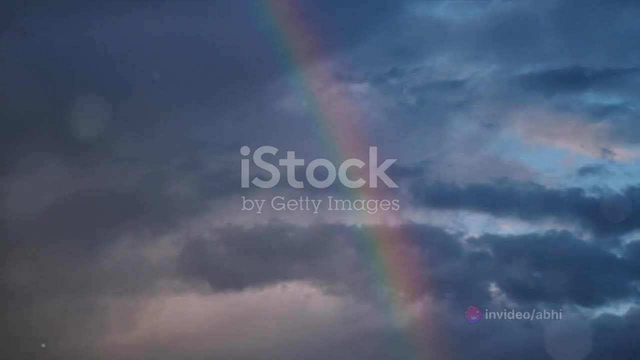 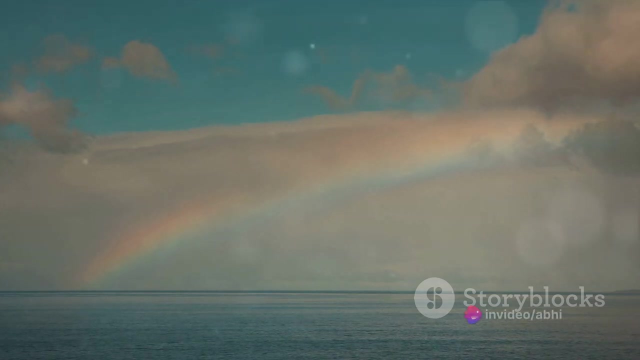 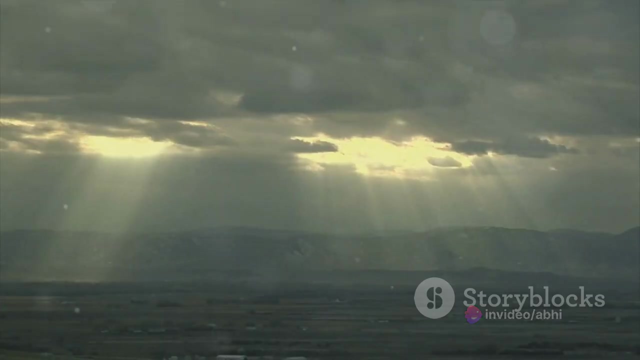 much further than this basic explanation. Light is a curious entity, a phenomenon that demonstrates properties of both a particle and a wave. This is a concept that continues to puzzle and fascinate even the most enlightened minds. Light, unlike typical matter or simplistic waves such as sound. 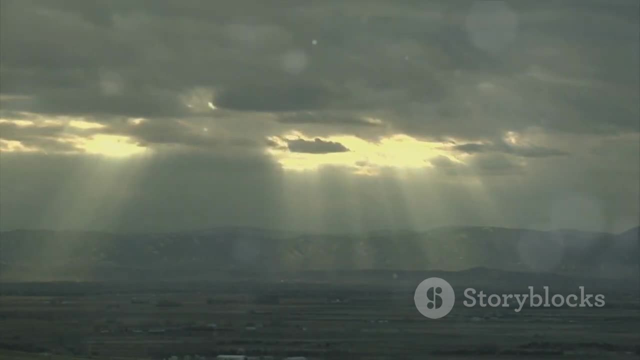 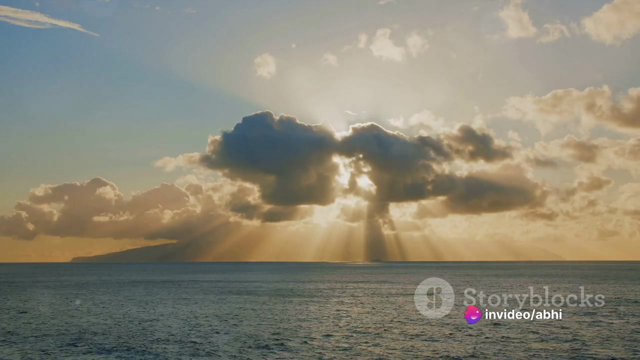 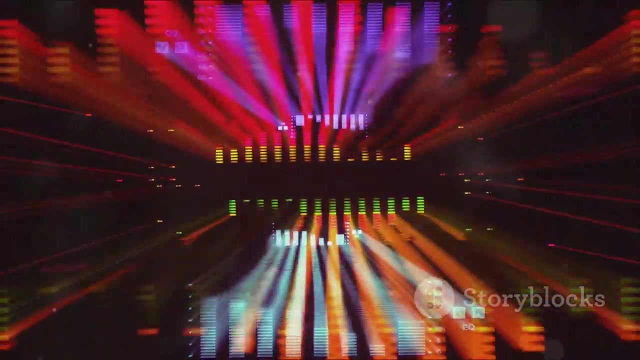 or water waves behaves distinctly. This enigma is referred to as the wave-particle duality, a fundamental principle of quantum theory. Understanding light as a particle means recognizing that it carries energy in discrete amounts, called quana. This particle-like behavior can be observed in phenomena like the photoelectric effect, where light illuminates a. 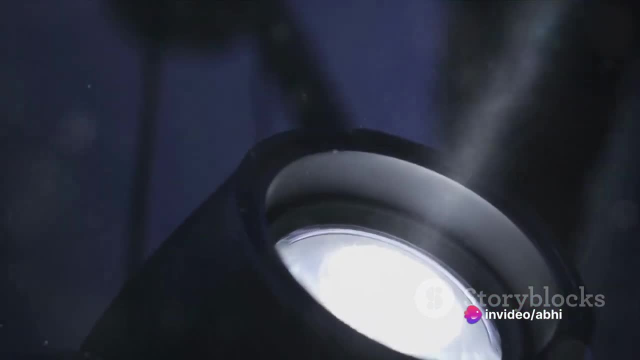 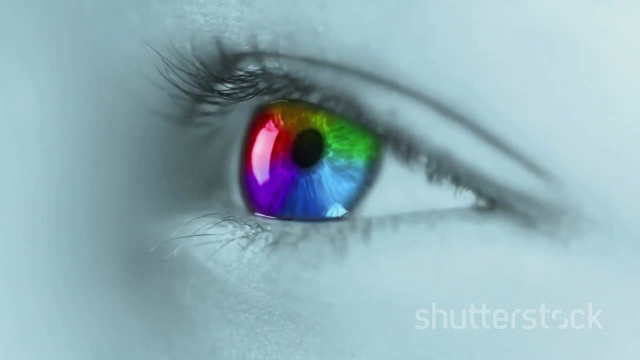 metal and ejects electrons. On the other hand, understanding light as a wave implies that it is a form of electromagnetic radiation that travels through space in a wave-like manner. This wave like phenomenon is a phenomenon that can be observed in phenomena like the photoelectric effect. 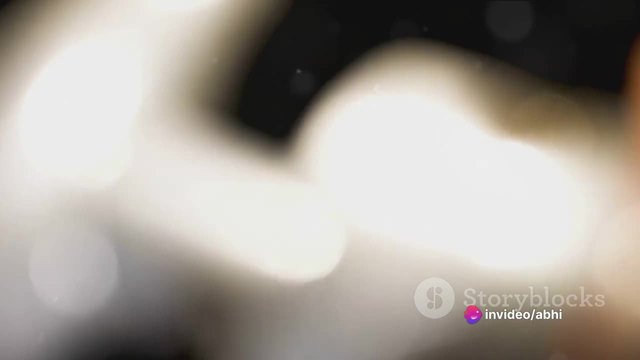 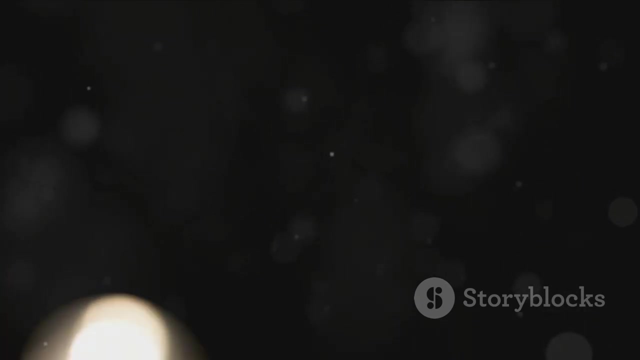 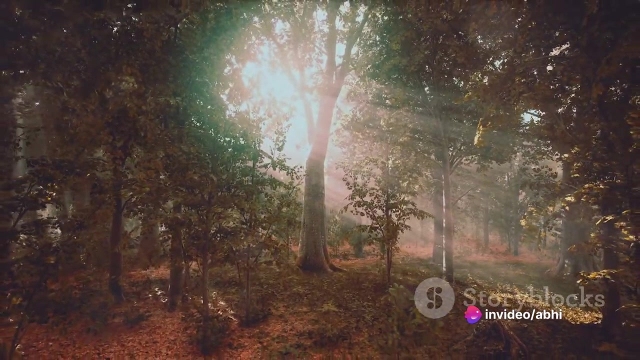 where light bends around objects. and interference, where waves of light can amplify or cancel each other. In the case of a sunrise, the stunning colors we witness are a result of the interaction between light and the Earth's atmosphere. This mesmerizing spectacle transpires dispersion of. 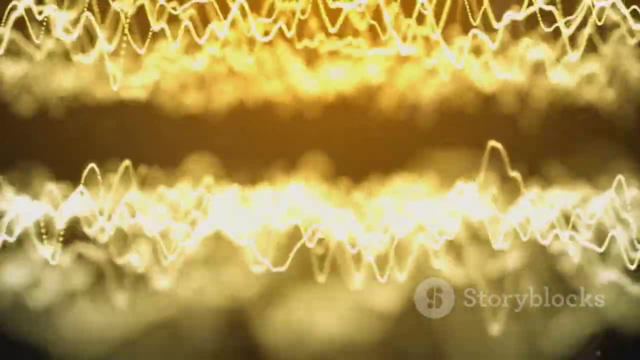 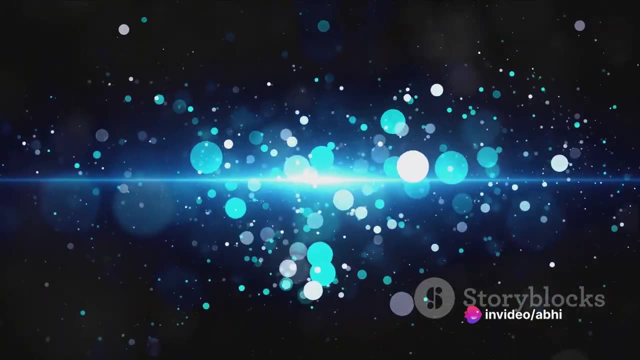 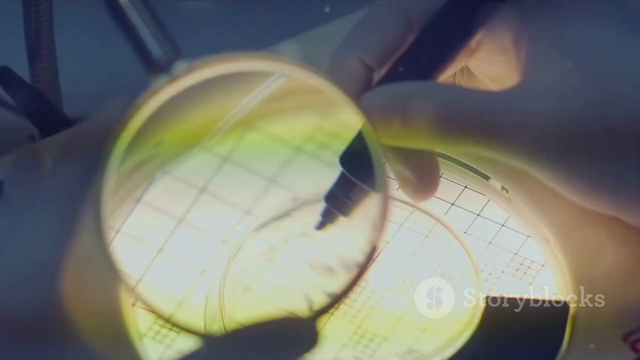 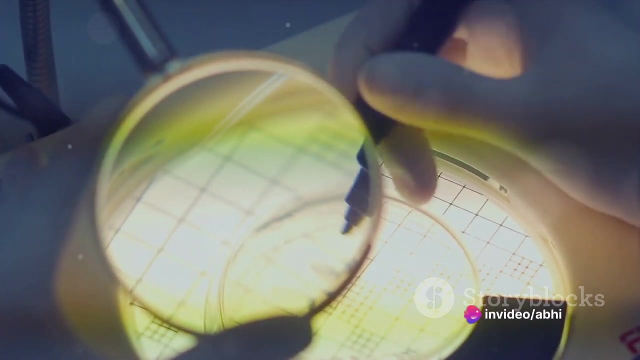 light scattering across the horizon in a harmonious display of colors. Regarding rainbows, they materialize when sunlight passes through rain droplets. Light's various interactions with the elements around us culminate in some of the most breathtaking marvels we behold. Light is an entity that, despite its omnipresence, continues to defy. 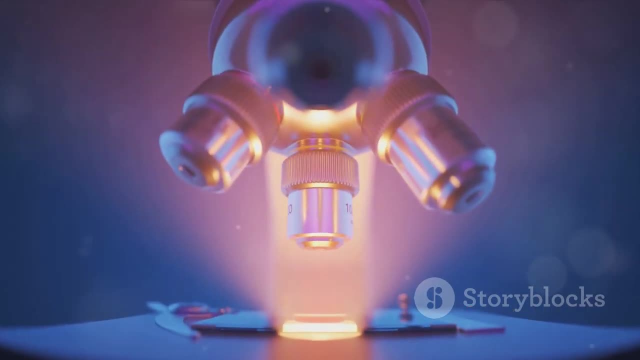 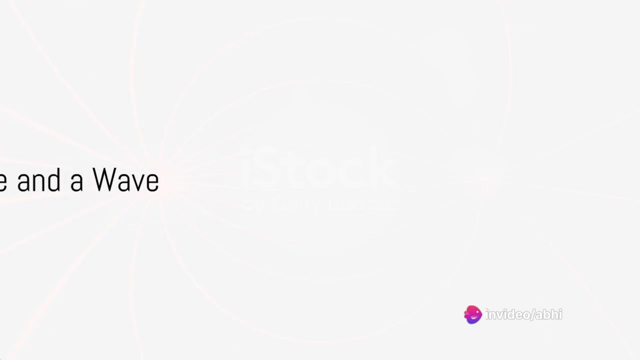 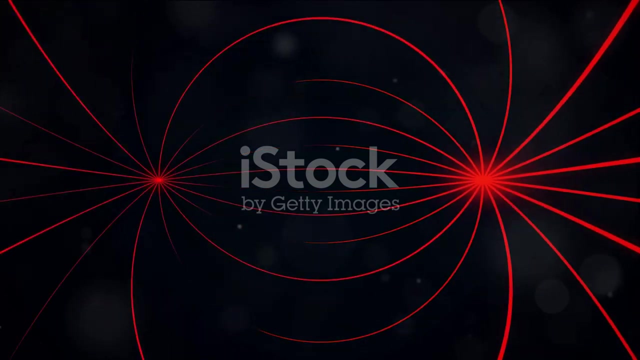 complete understanding. This intriguing phenomenon, being both a particle and a wave, is a concept that even the greatest minds have grappled to fully comprehend. Indeed, the concept of light as a particle is a fascinating one. At the heart of this concept are tiny packets of energy we refer to as photons These minute. 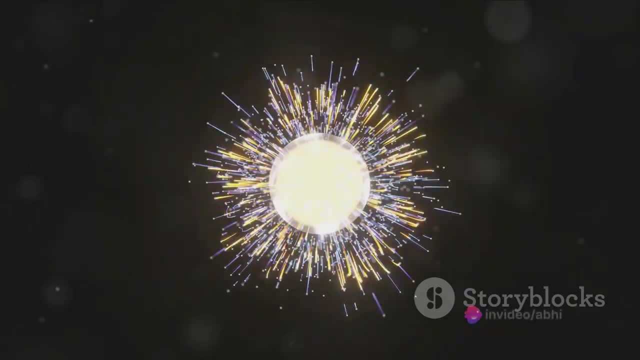 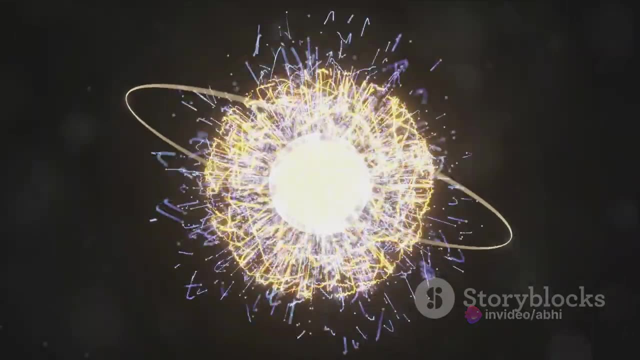 bundles of energy. these photons are a marvel of the natural world. They traverse space in a straight line, unwavering and resolute, undeterred from their chosen path. It's as if they've been shot straight from a laser pointer, cutting through the vast expanse. 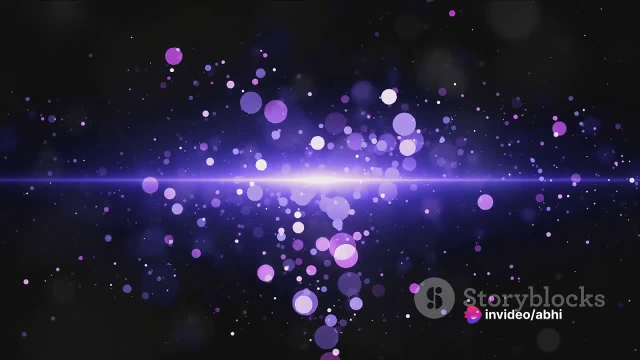 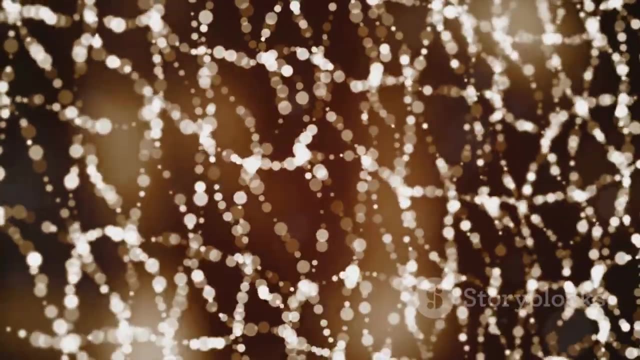 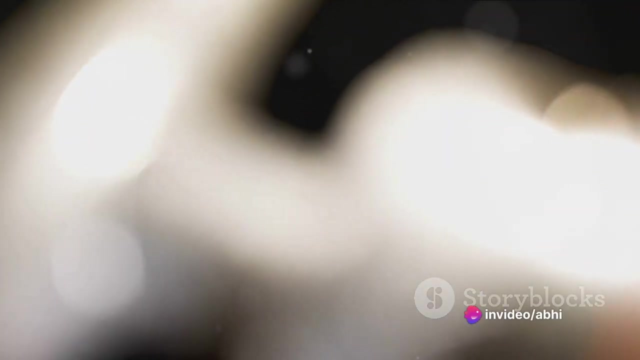 of darkness like a samurai sword. The steadfast persistence of photons is truly remarkable, but their journey does not stop when they meet an obstacle In their path. rather, they interact with the material, either being absorbed into it or changing their course. This interaction results in one of the most mundane yet intriguing aspects. 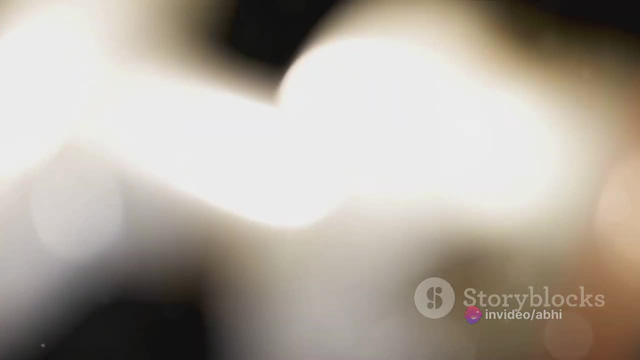 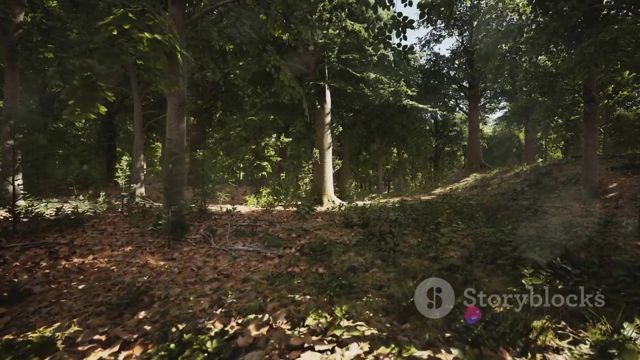 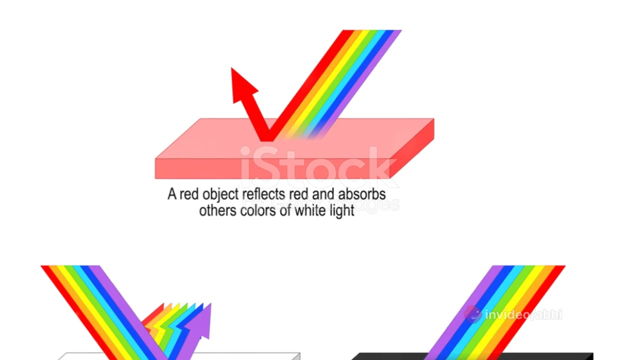 of our lives: the formation of shadows. Shadows are a stark contrast of darkness in the presence of light, a result of objects blocking the determined path of photons. Phenomenas such as shadows are not the only interesting aspects of. They also help explain why our eyes perceive. 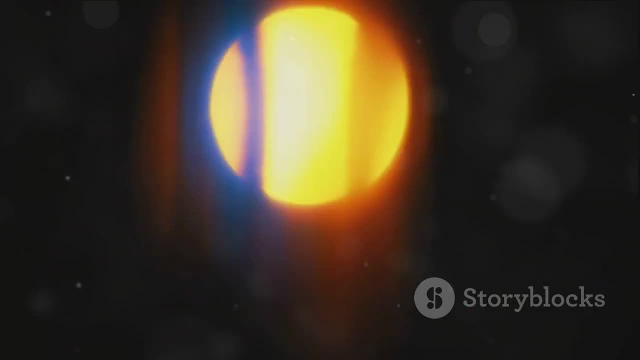 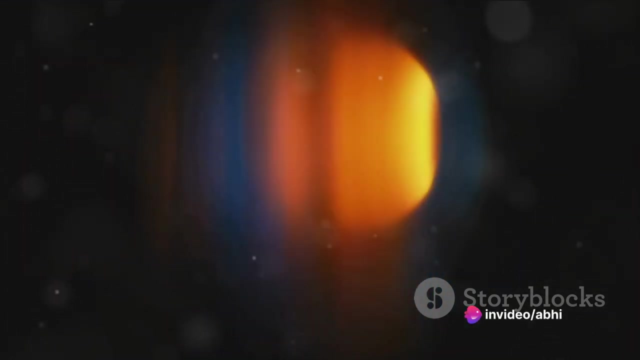 objects in different contexts. For instance, if you're looking at a red apple, it's not essentially red. Instead, it's absorbing all colors of light except red. The photons reflecting this unabsorbed red light reach our eyes and we perceive the apple as red. a simple yet fascinating 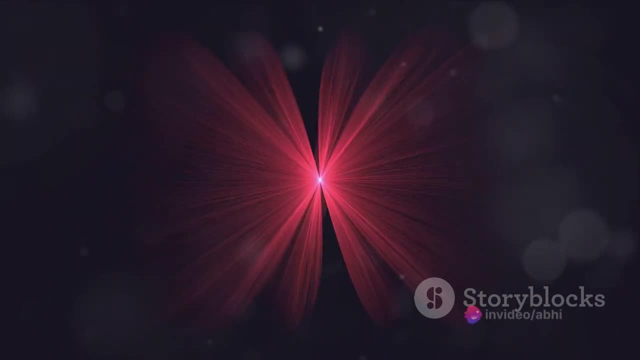 explanation of colors. Conversely, light is not just a stream of tiny packets of energy. It also has wave-like properties, mimicking the uniform spreading ripples on a calm pond. These waves, determined by their length or wavelength, come in varying sizes. They are 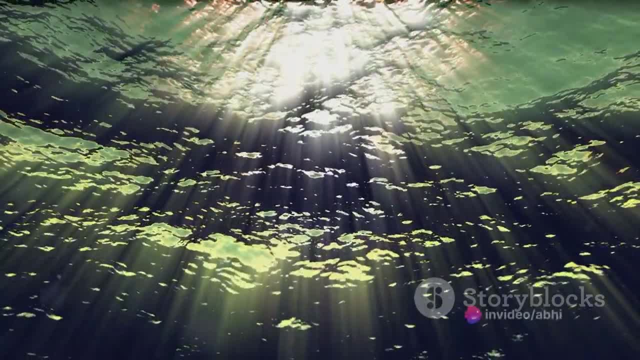 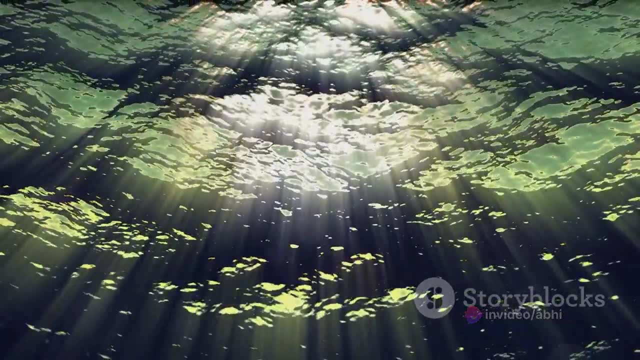 different in color, color and color diversity In our visual spectrum. they are both located in a distinct color. Shorter waves are perceived as blue or violet, while longer waves are seen as red. But the wave properties of light are not just responsible for the colors we 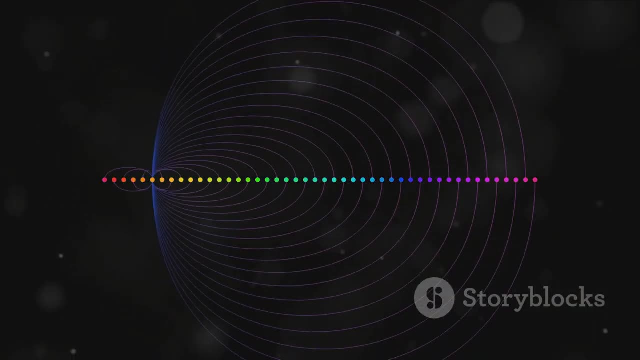 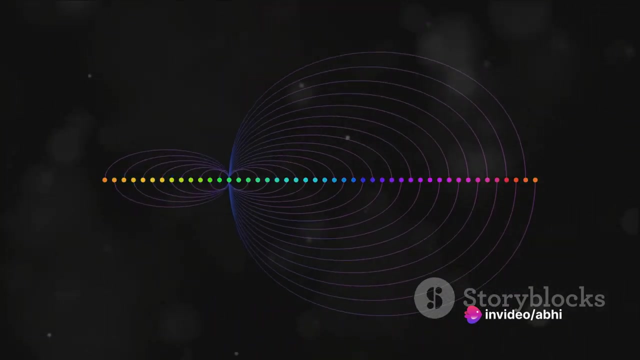 see, They are also behind another captivating phenomenon known as diffraction. This is the reason light can bend around corners, finding its way into spaces and corners where you wouldn't think it possible. It's the wave property of light that allows diffraction to happen. 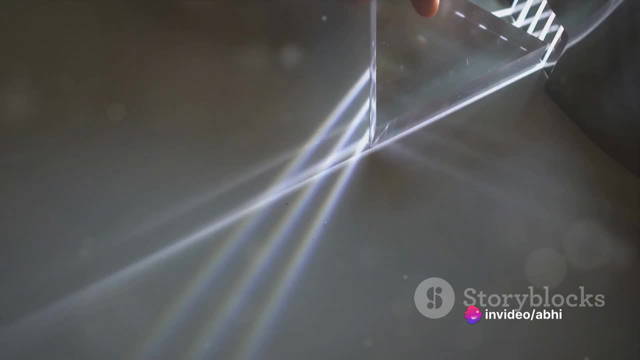 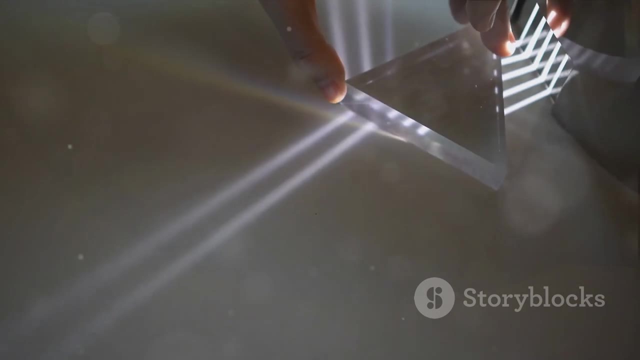 to reach places beyond direct line of sight, just like how sound waves can travel around corners. this dual nature of light, its ability to behave both as a particle and a wave, continues to bewilder and amaze and layman alike. light, apart from illuminating the world, possesses. 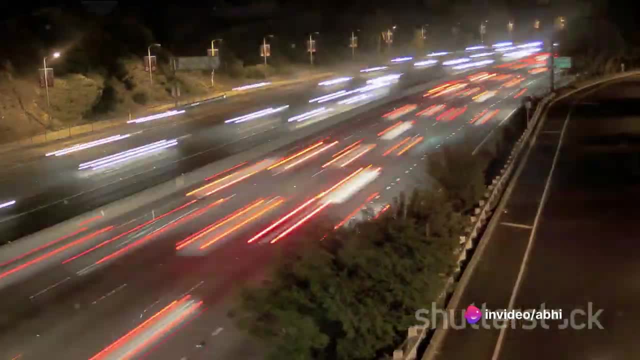 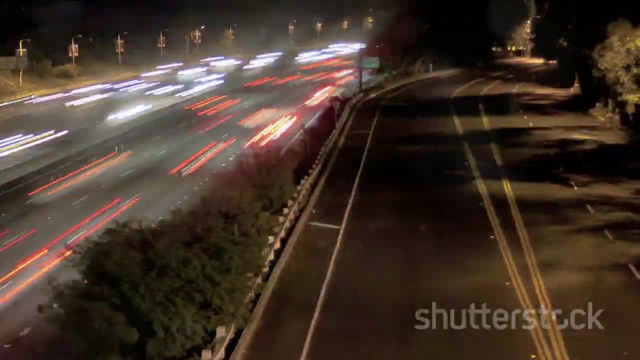 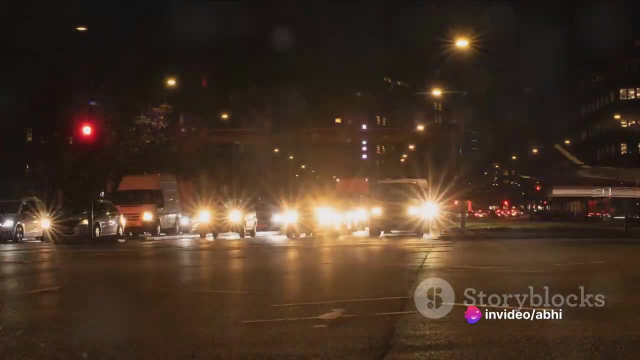 two key features that are truly remarkable: its astounding speed and a phenomenon known as polarization. the speed of light, a staggering 200 000 miles per second, is a marvel that continues to astonish scientists and scholars around the globe. this speed is so vast and overwhelming that 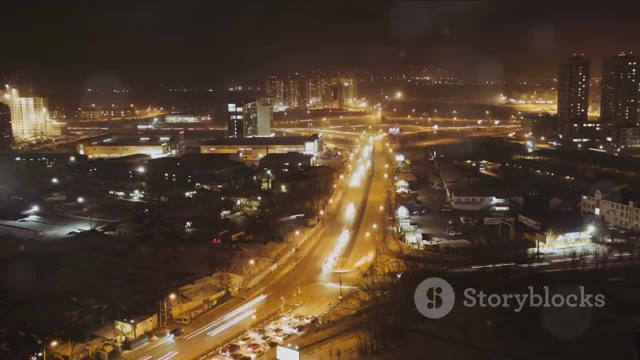 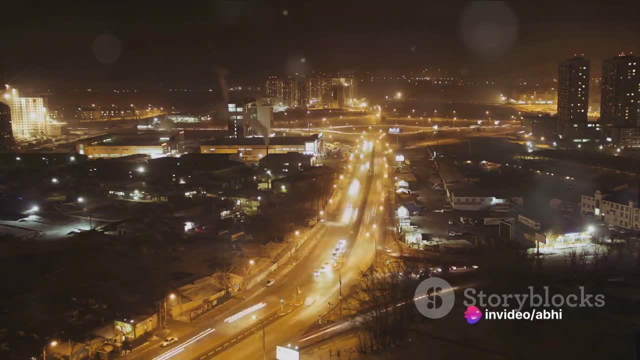 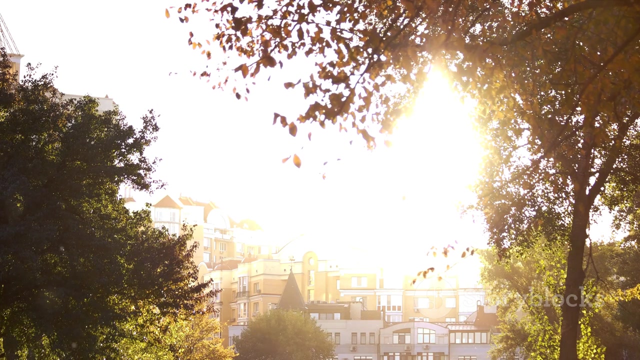 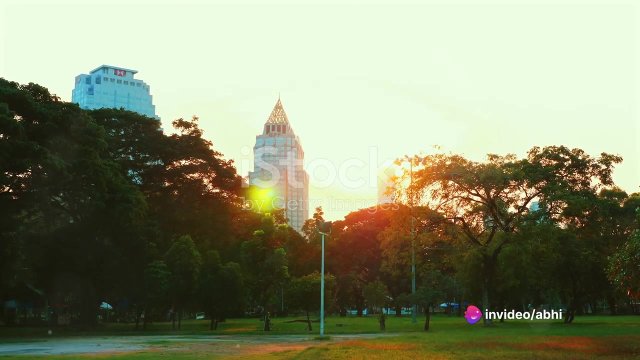 it surpasses our human understanding. to illustrate this, consider our own sun, the fiery celestial body that is approximately 93 million miles away from our place of residence. earth, at the breathtaking speed of light. sunlight requires a mere eight minutes to travel this colossal distance and reach us. imagine that only eight minutes to traverse a distance of over 93 million miles alongside 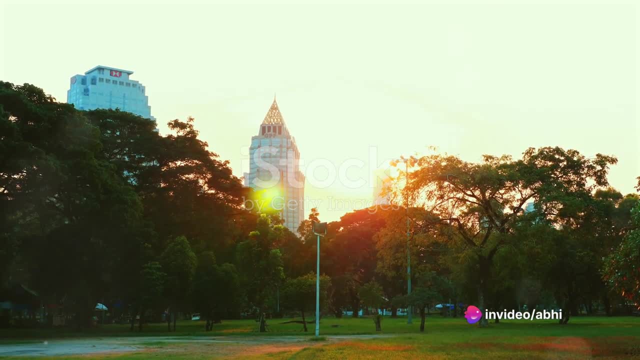 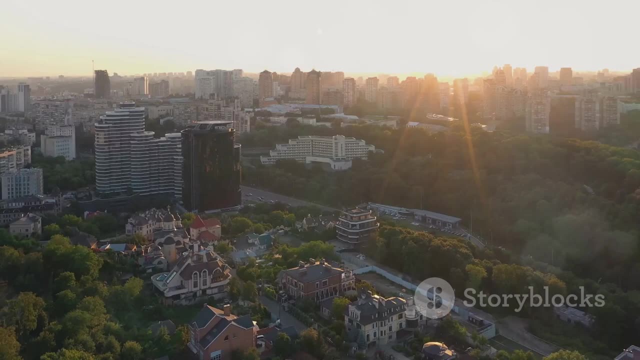 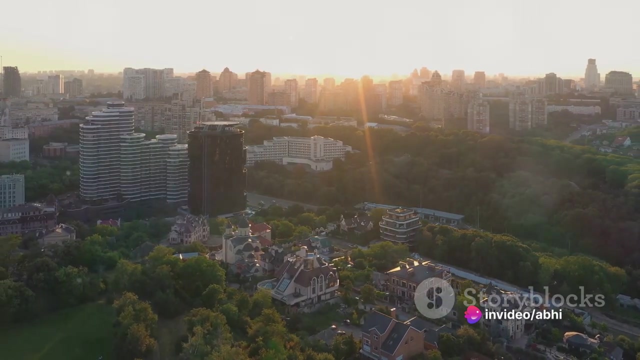 its incredible speed, light also exhibits another fascinating characteristic: polarization. this property signifies that light waves have the potential to vibrate in multiple directions. this aspect of light is indeed captivating and has practical implications in our day-to-day life. ever pondered why specific sunglasses are so proficient in reducing the irritating glare? the 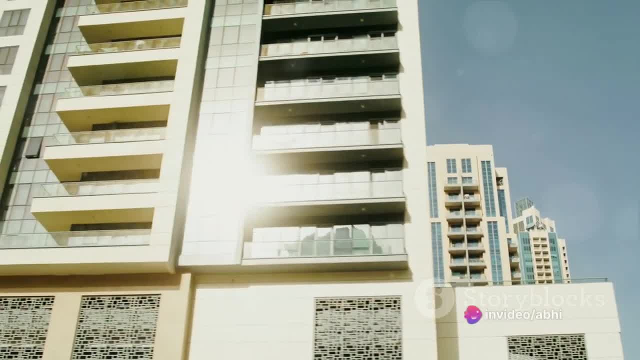 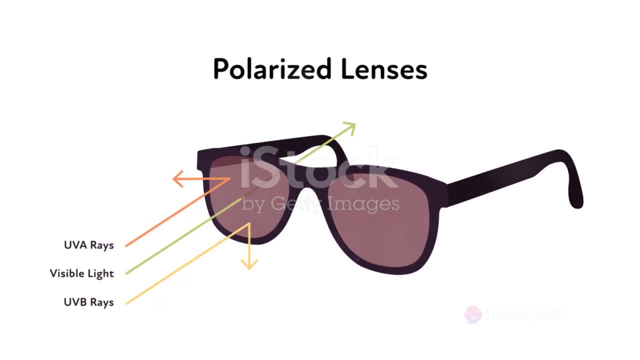 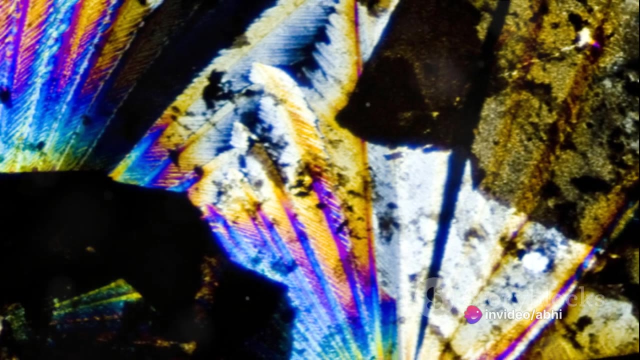 answer lies in the polarization of light. these sunglasses act as a filter, blocking light waves in certain directions and consequently reducing the glare. this application of light's polarization makes our everyday lives more comfortable, especially on sunny days. the concept of light speed and polarization also plays a crucial role in telecommunications. it allows our telecommunication. 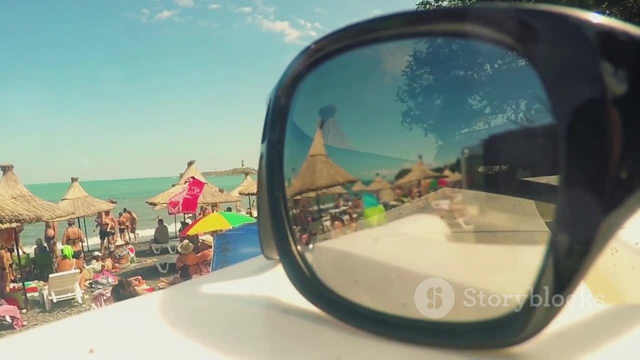 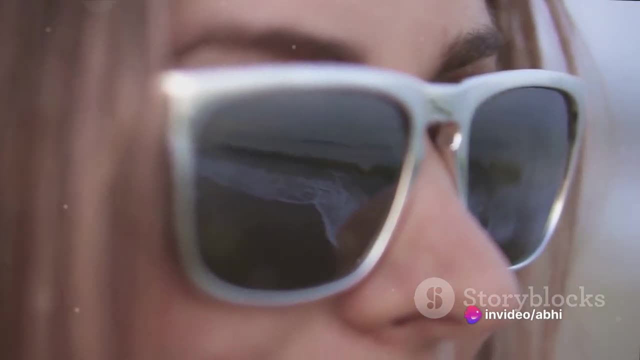 devices to send and receive data at high speeds, enabling us to communicate with people halfway across the globe in real time. moreover, the phenomenon of polarization is also essential in the functioning of lcd screens. the lcd screens can be used to control the amount of light passing through each pixel. 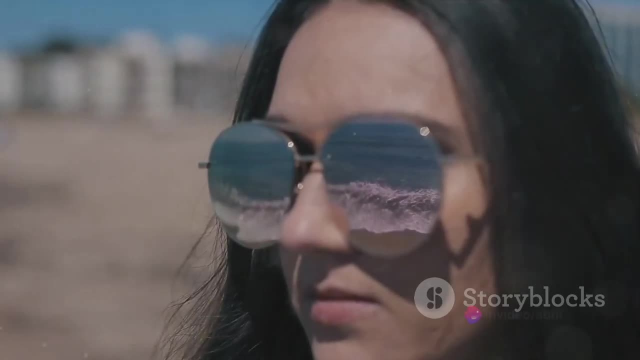 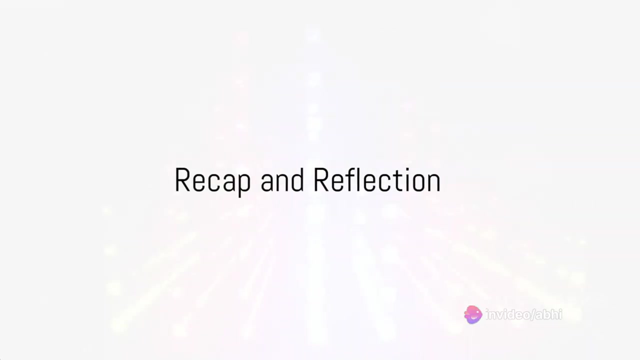 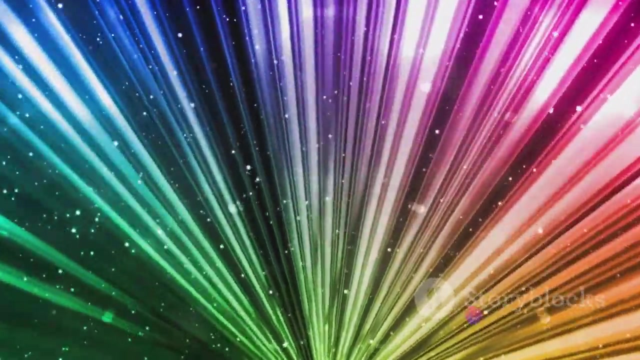 so every time you're watching your favorite show or texting a friend, remember it's the wonderful properties of light that are making that possible. in review, light is an extraordinary type of energy that uniquely behaves both as a particle and a wave. it journeys in straight, linear paths and is frequently absorbed or reflected when it encounters various objects. 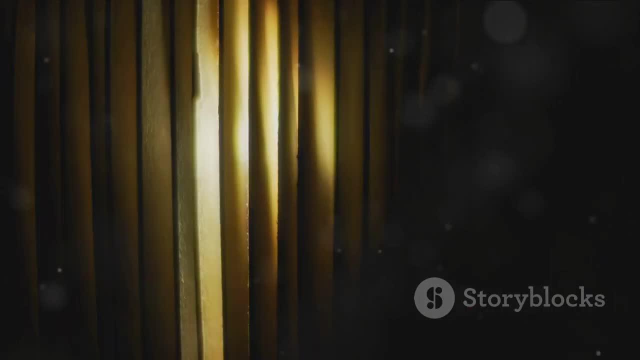 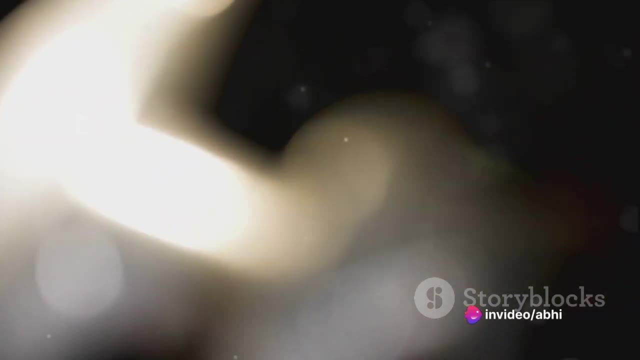 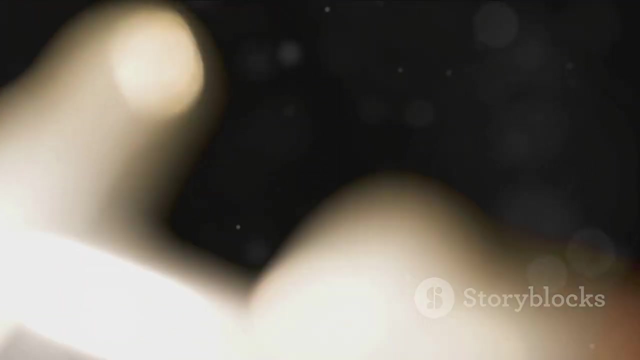 the distinct color attributes of of light are a direct function of its wavelength. this magnificent form of energy propels at an incredibly swift pace, approximately 300 000 kilometers per second. the speed of light is so rapid it almost defies comprehension. additionally, light's motion isn't confined to a single plane. it vibrates in of.